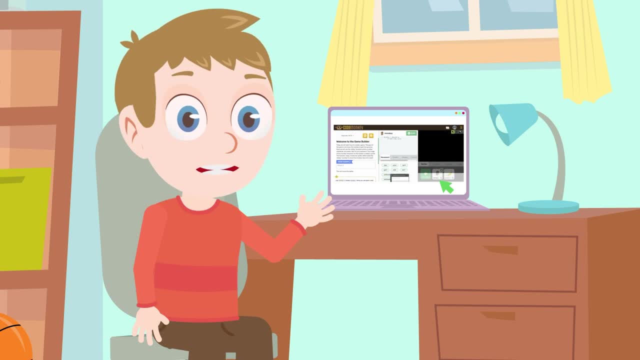 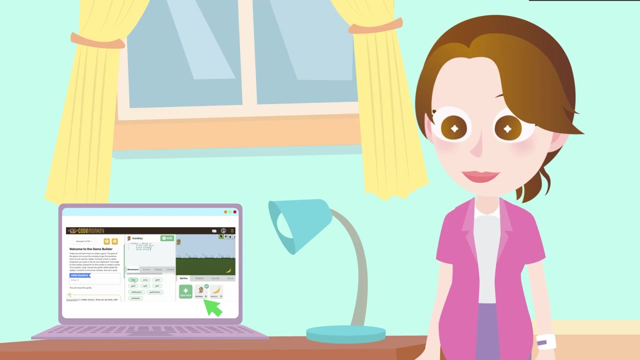 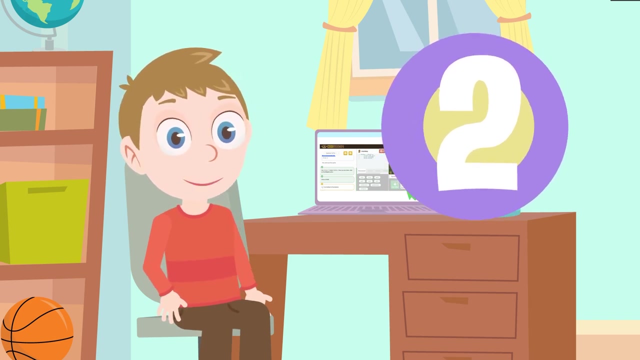 what I thought about programming language and how it works. Let's take a look at some of the things about programming language in Minecraft. Reason number two: Minecraft can be enhanced by modifications or mods that are outside strings. Minecraft has a unique design with provides for all kinds of coding You can. 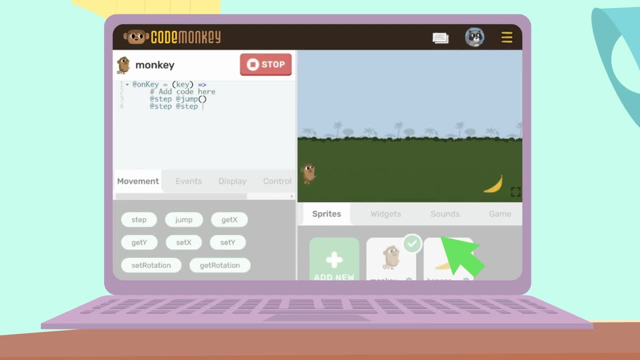 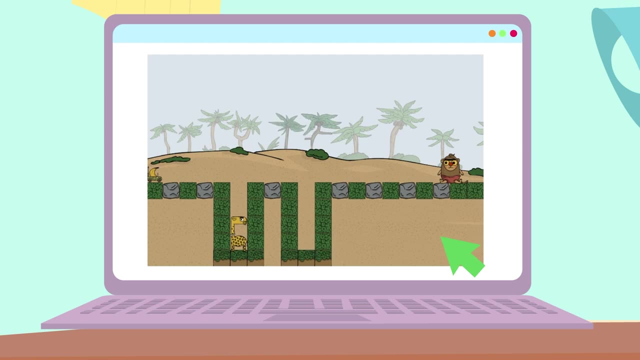 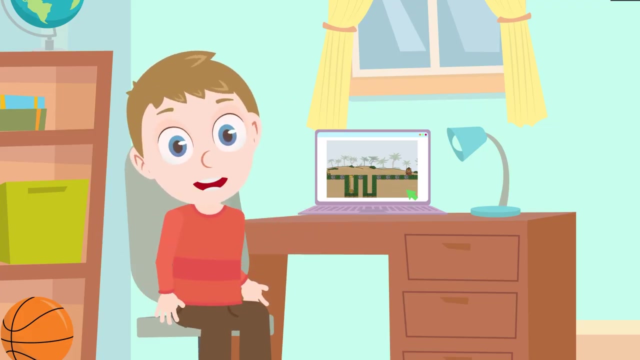 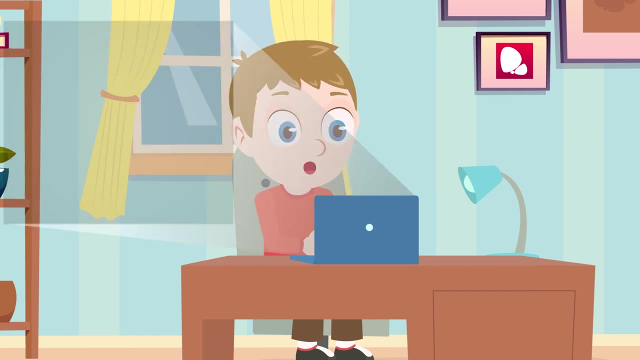 of code that change the game from the inside, such as generating monsters, giving players increased health or items and even telling the non playable characters to do specific things. I have been working on building some of these mods by writing my own code, and there are even block based programs out there that. 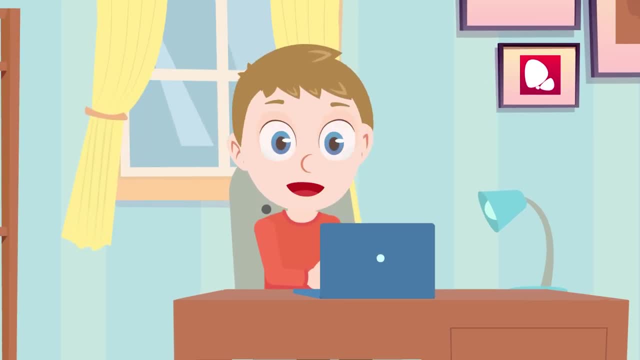 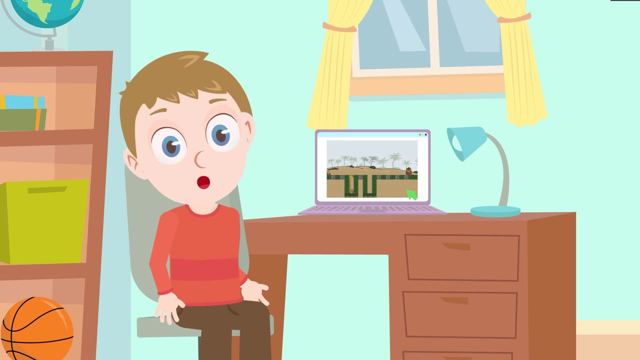 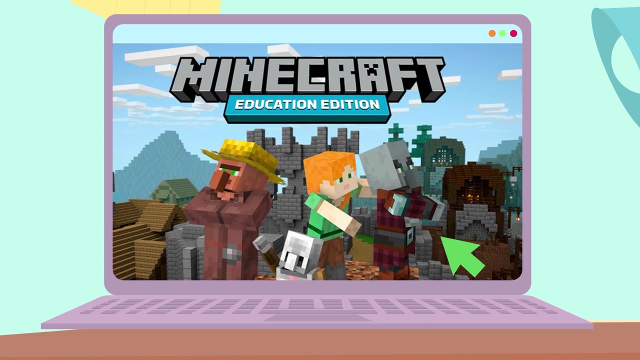 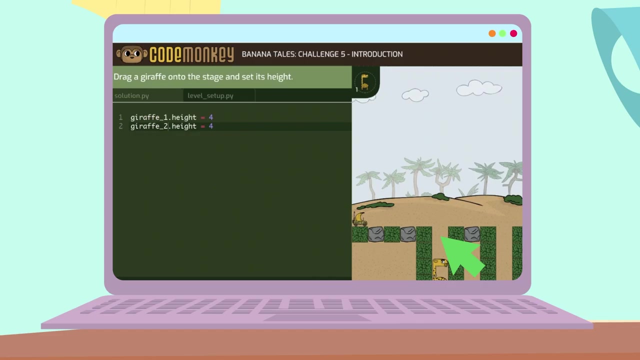 can help with these as well. so I am learning to code and I'm playing at the same time- win-win. Reason number three: Minecraft even has an education edition. we sometimes use it in school. coding languages often involve a lot of strings of words, numbers and letters, meaning that more complex coding 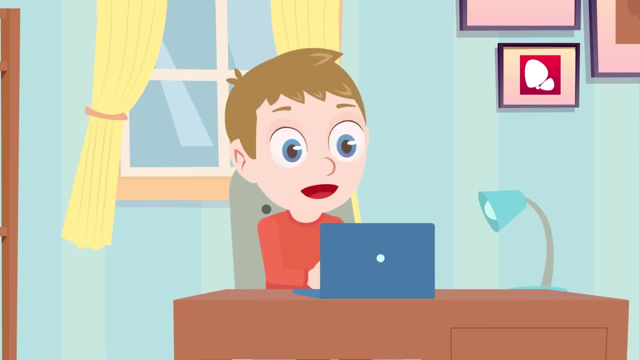 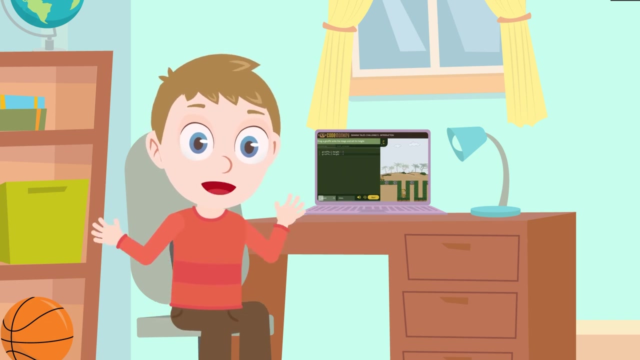 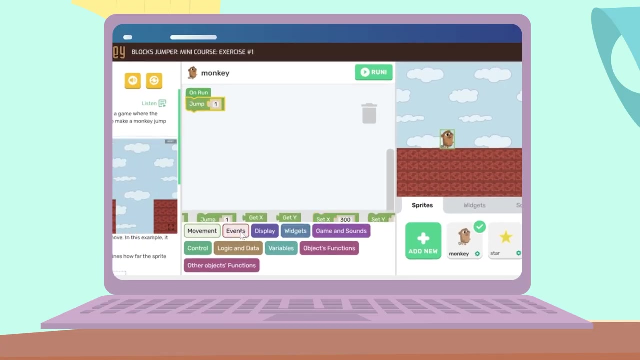 involves more complex coding, a lot of typing. This can often seem daunting to children and to people who aren't very confident with typing very quickly. However, programs such as Minecraft Education Edition offers a far more visual and less wordy way of learning to code as a beginner by using visual block coding. This 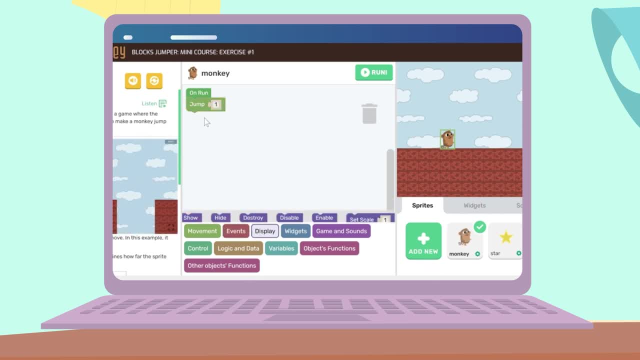 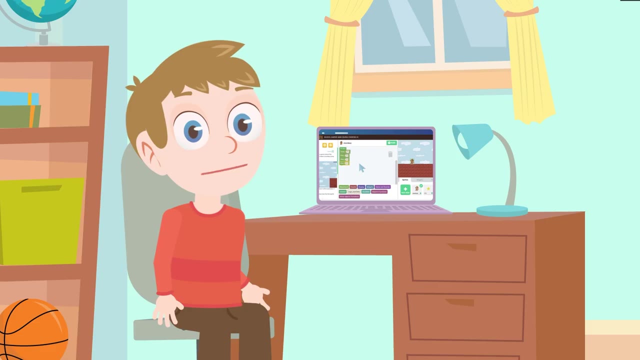 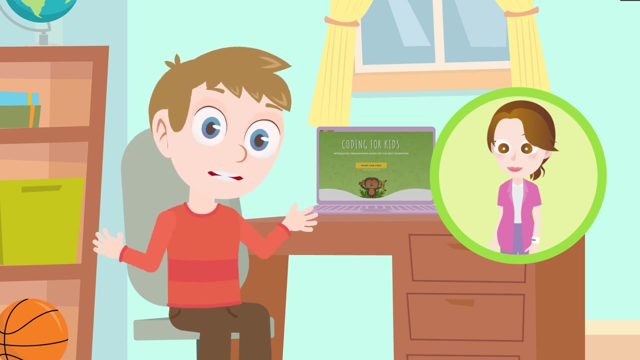 involves individual blocks of pre-written code that can be dragged and dropped into the script just like a puzzle piece. This helps us understand the coding format and how we can change elements in a game in real time. Mum. why don't you try So, mum? as you can see, Minecraft is a very important. 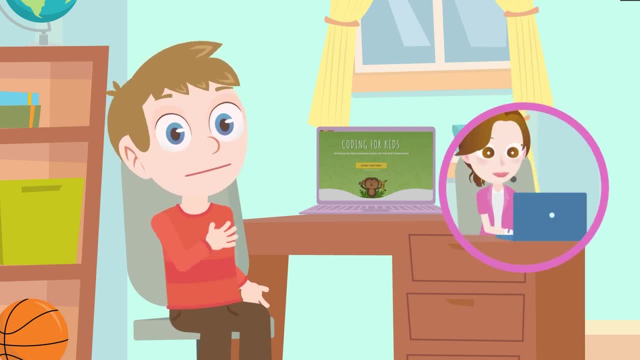 tool on my coding journey. Mum, now it's your turn.